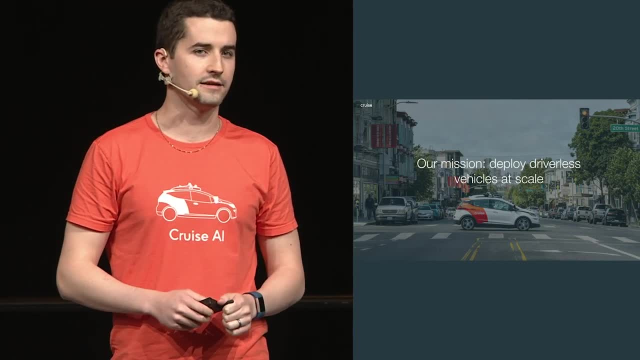 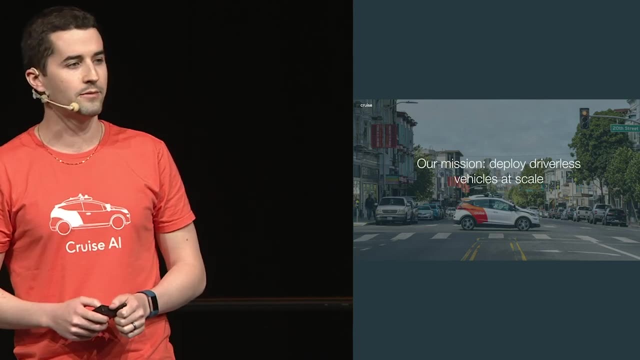 So being part of self-driving cars is a really exciting mission. whether it be just making your average commute a little bit more enjoyable, or giving mobility back to people who need it, or, ultimately, saving lives, It's a very rewarding mission to be a part of. 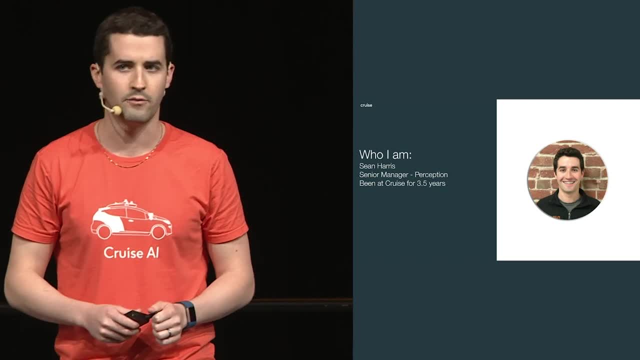 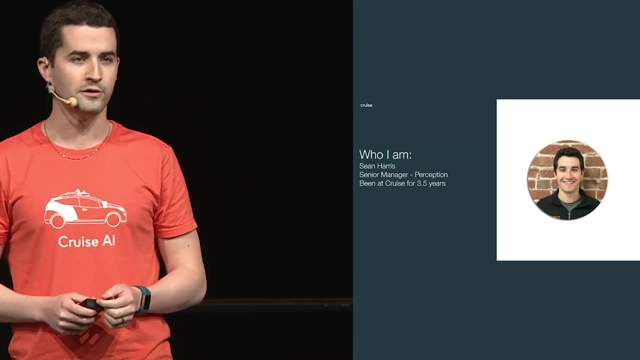 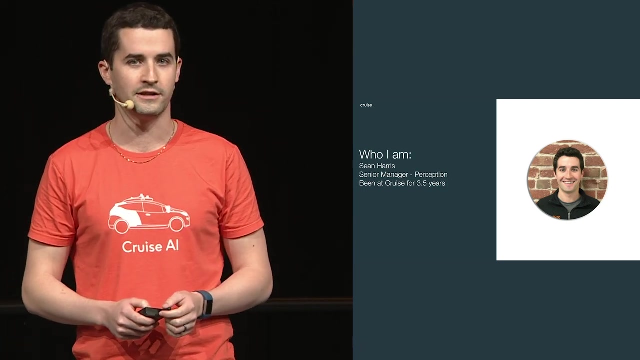 I'm an engineering manager for the perception team at Cruise. I did a PhD in reinforcement learning. I've been doing ML and robotics for about eight or nine years now, And I've been at Cruise for about three and a half years, And so I'm excited to take you through what solving machine learning problems at Cruise is like, because I believe that the future of ML really lies within autonomous vehicles. 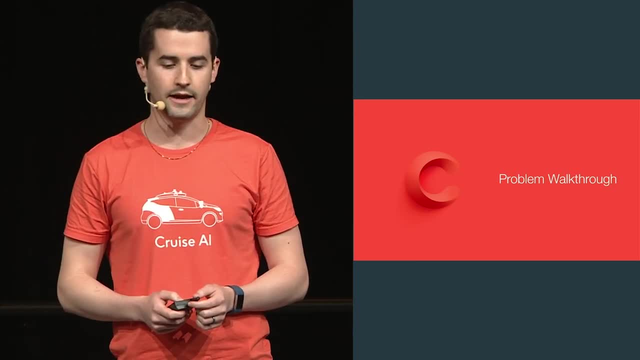 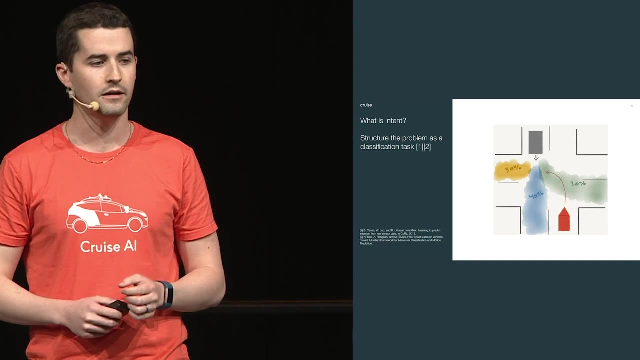 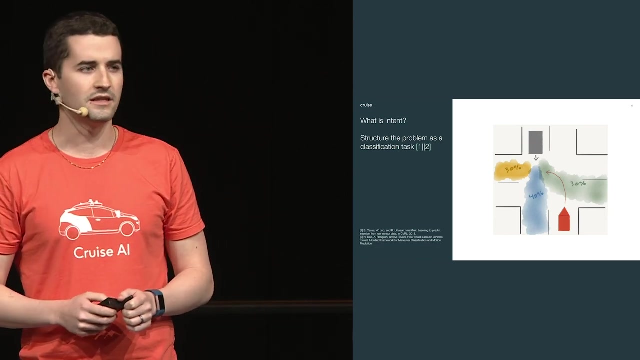 Okay, so let's start with the problem. The problem I want to walk through with everyone today is called prediction. We talk a lot about object detection in literature, but prediction is equally exciting and if not more challenging. So the problem we're trying to solve in prediction is: we're trying to understand what does another agent in the world? 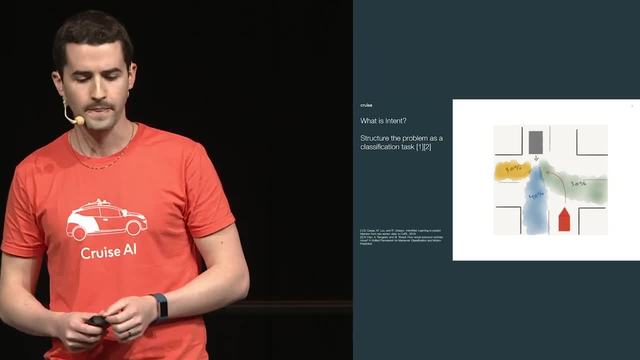 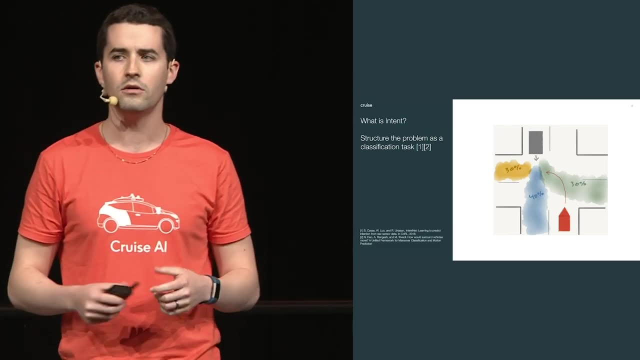 want to do in the future. Where are they going to go? And because we only have 20 minutes, I'm going to simplify the problem a little bit. We're just going to talk about intent At a high level. where does another agent want to go? What do they want to do? 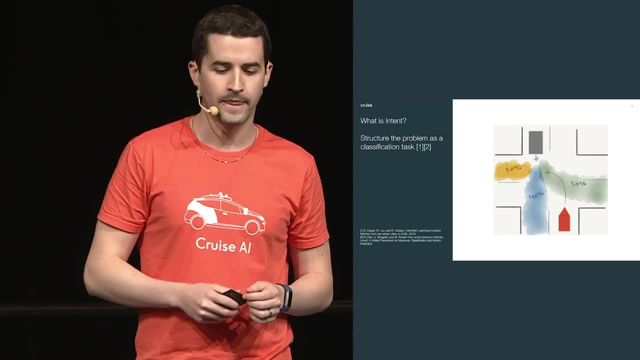 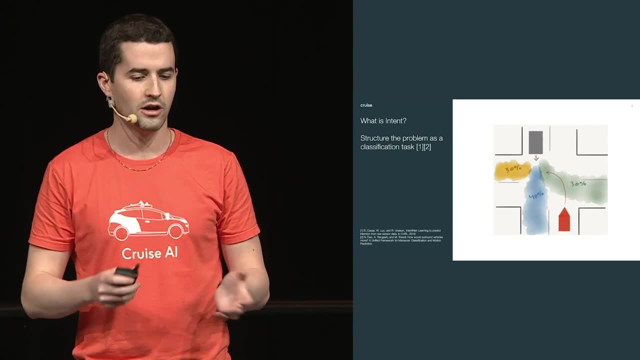 We're not so worried about how they're going to do it, just about what they want to do. And so in this example that I have here, maybe the cruise car is in red and there's an oncoming car and we're trying to understand: what do they want to do? Are they going to go straight? Are they going to turn left? Are they going to turn right? 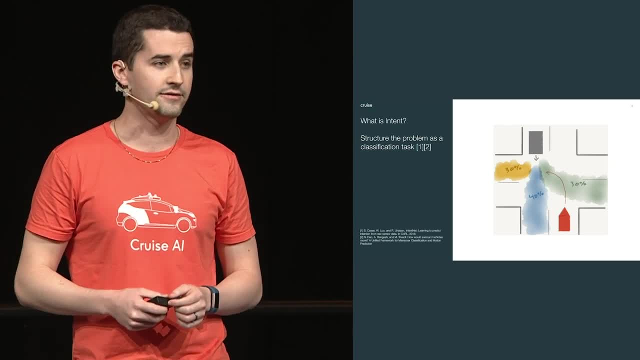 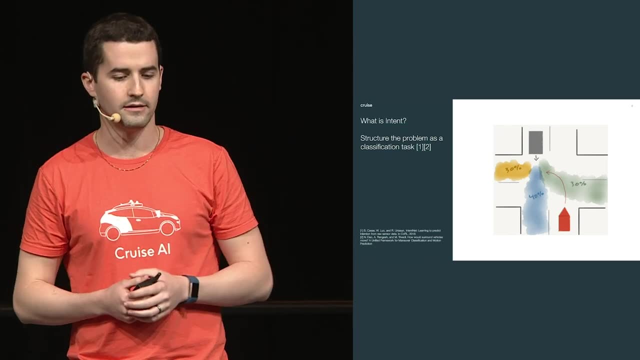 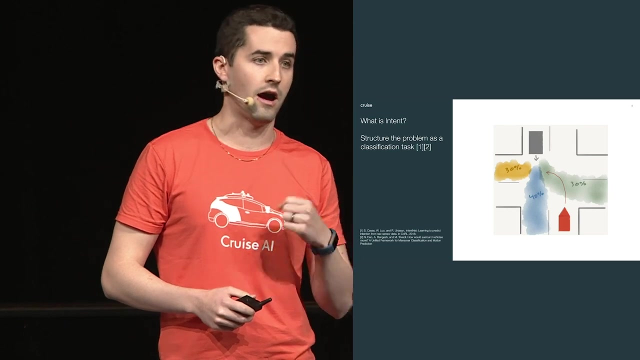 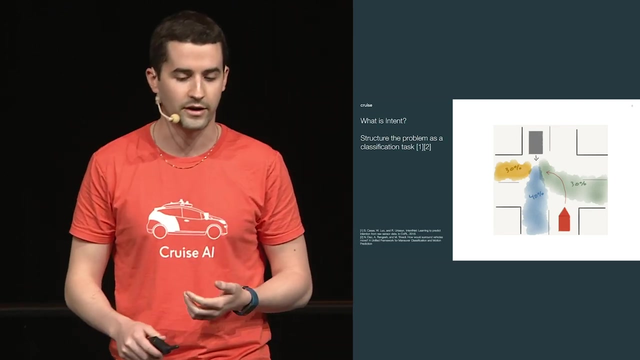 And so we can structure this as a classification problem. We can come up with a bunch of different actions that can all be our classes. There's a few different papers that use this kind of problem- representation- And then the input to this task is basically the state of our object that we're trying to predict. So it's position, it's velocity, it's type. so is it a car or a truck, or a bicycle, or a pedestrian? 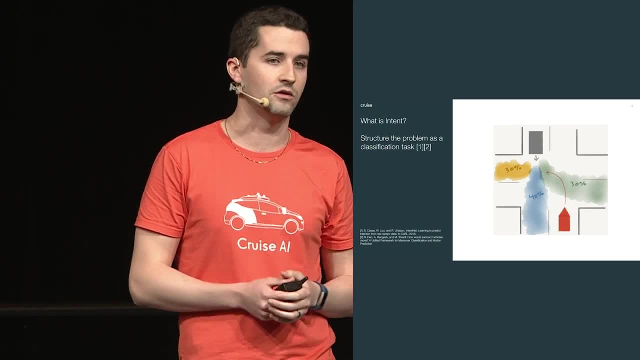 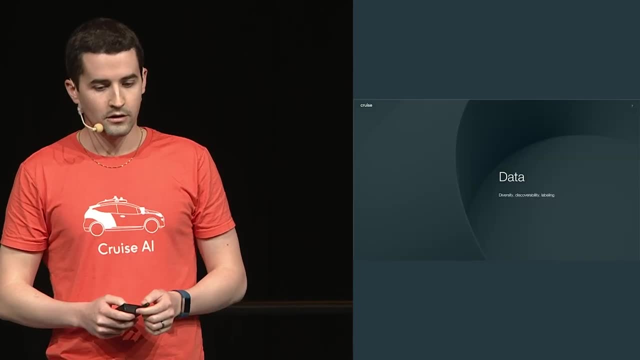 It's shape, maybe it's orientation and where it is in the world, And what we're trying to do is understand what is it going to do in the future? So, like any good ML engineers, let's start by looking at the data. 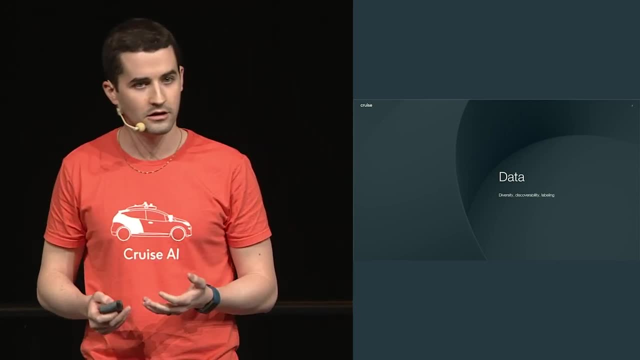 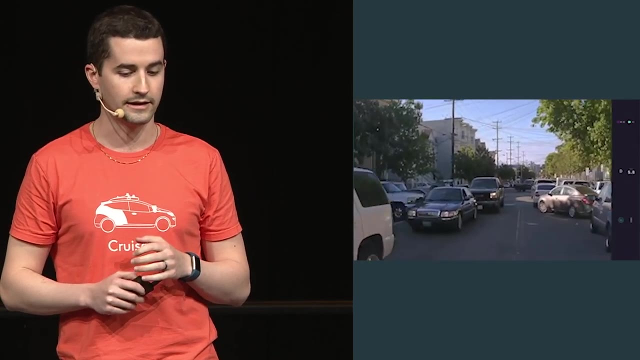 So we want to build data sets that are large and diverse. Cruise has over 100 cars that drive around downtown San Francisco and collect lots of data. That's very exciting. Here is our car trying to navigate the perils of school dropouts. 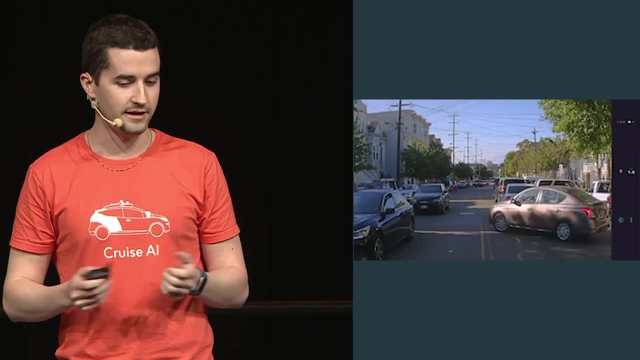 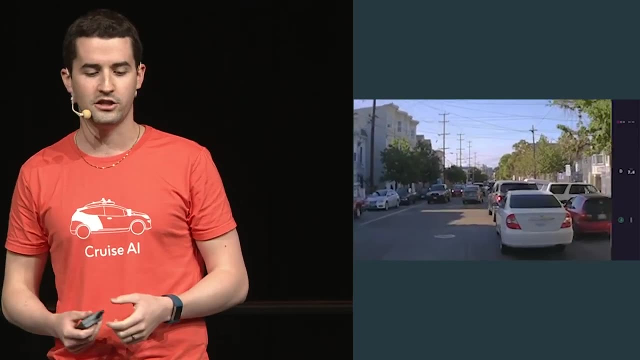 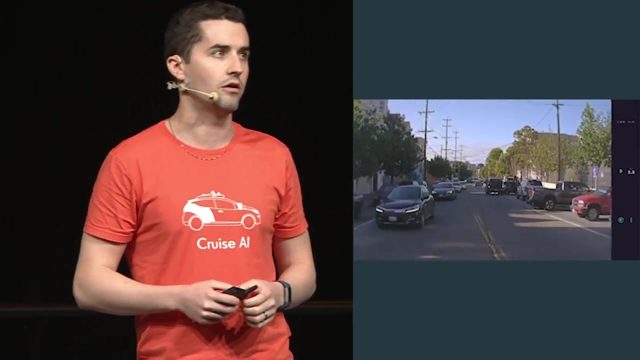 We have a lot of traffic in San Francisco which, as you can see, is full of a lot of kind of chaos around. the exciting thing about driving in an open environment is, although it's very challenging, we get exposure to very exciting and very unique events that you don't see much of on a highway or in a very quiet residential neighborhood. 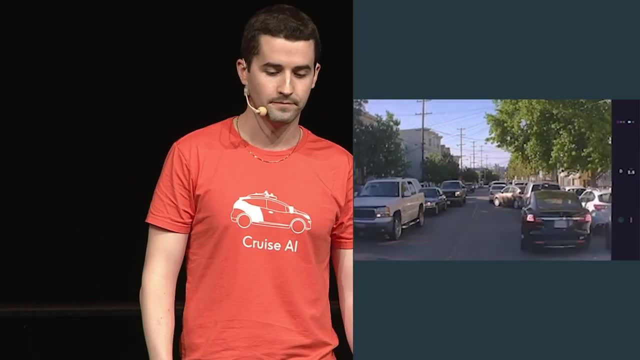 So we build very large data sets, but also very diverse data sets as well. It's not just about building a good data set, though. We have to really understand how to build a good data set. We have to really understand how to build a good data set, though. 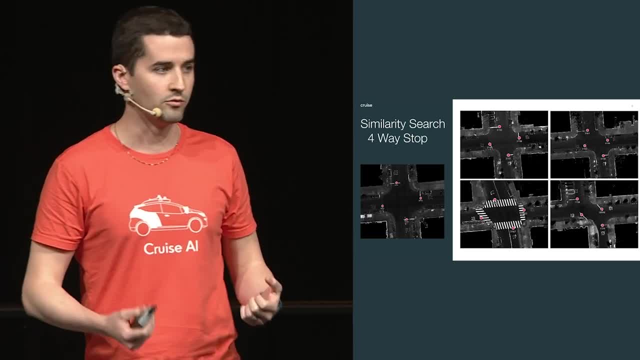 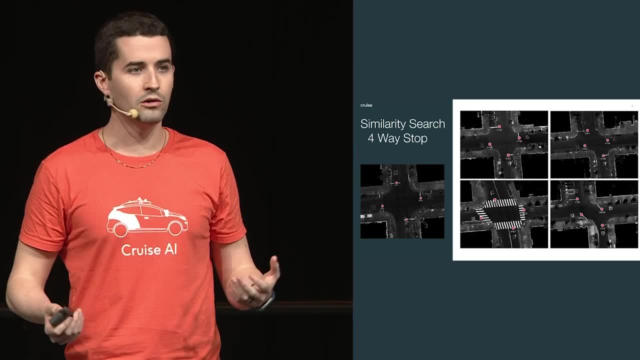 We have to really understand how to build a good data set, though. We have to really understand how to build a good data set, though, We have to really understand our problem and our data deeply in order to train a good model. And so, using our example of a car at a four-way stop from before, if we go and look at all the different four-way stops in San Francisco, it turns out there's a huge variety of different four-way stops that we see. 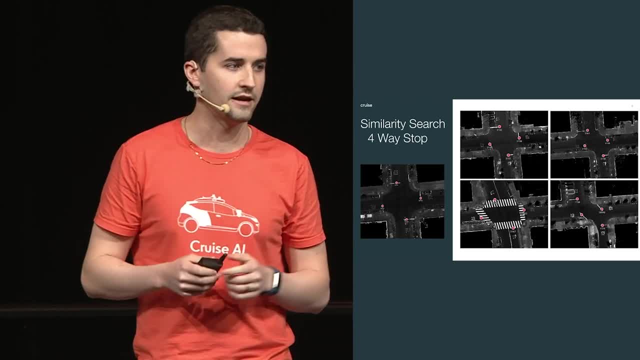 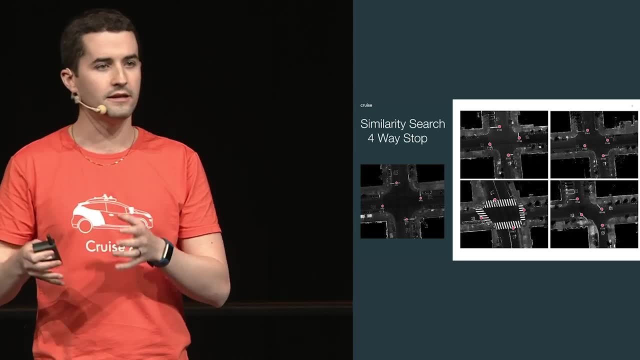 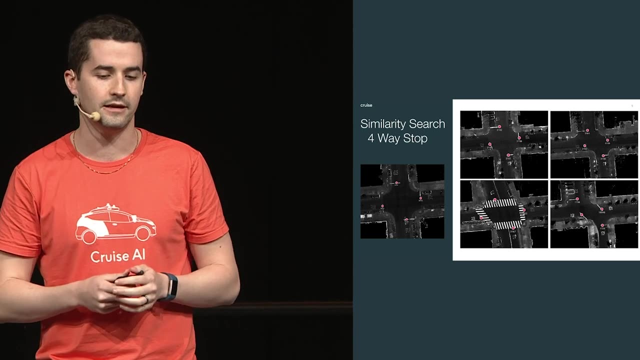 On the far left is a nice four-way stop where it's sort of nice and T-shaped and very uniform, And then on the right-hand side there's a variety of increasingly kind of wonky intersections where there are still four-way stops But they're not nearly as square or sort of T-shaped as the others. 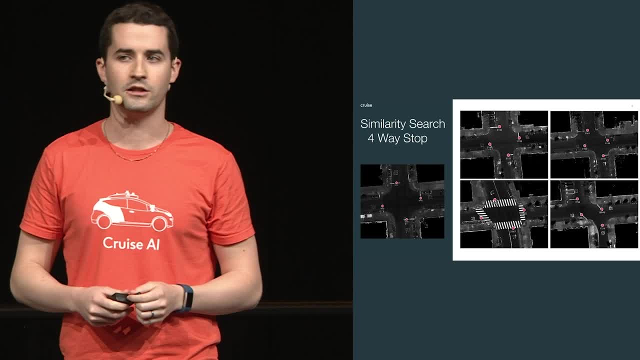 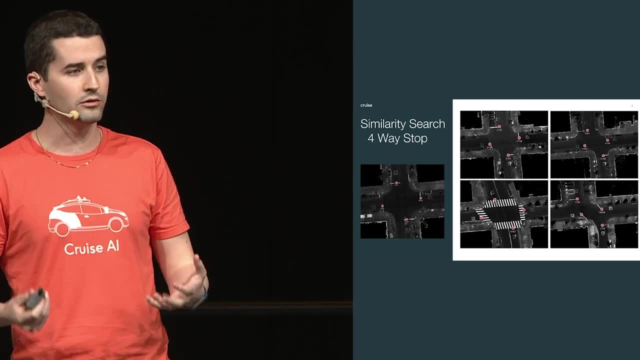 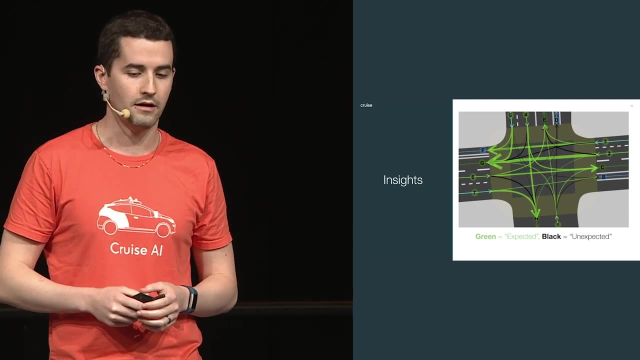 And so it's important for us to be able to understand these insights so that we can craft our model well and deal with all these different edge cases. So we invest a lot in the tooling to make this kind of thing easy to discover. Some other insights that we might gather is around how much people behave as they are supposed to on the road. 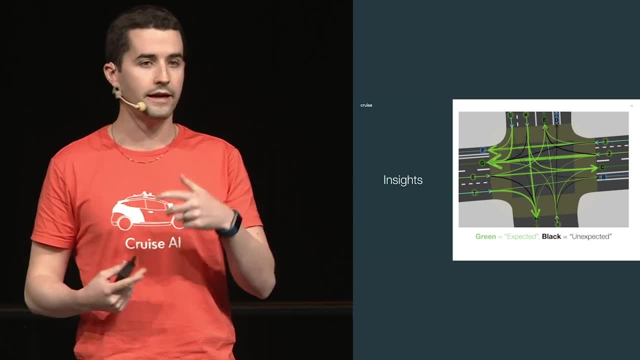 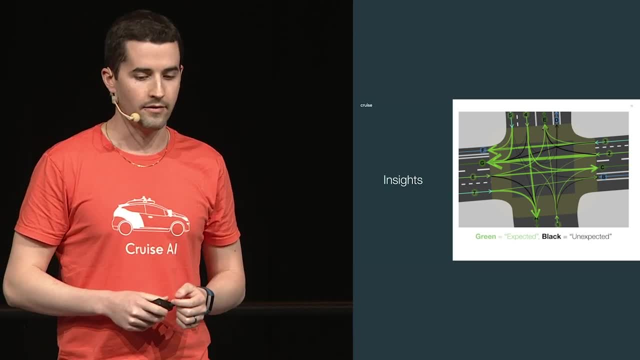 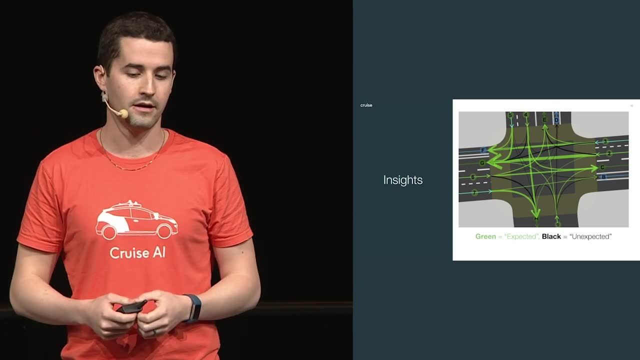 So this is a different four-way stop with one car lane, And this is a separate lane in every direction and also a bike lane in every direction, And the green represents what we, when a car does a maneuver that we expect it to do, And black is someone doing something that we don't expect them to do, based on sort of following the laws. 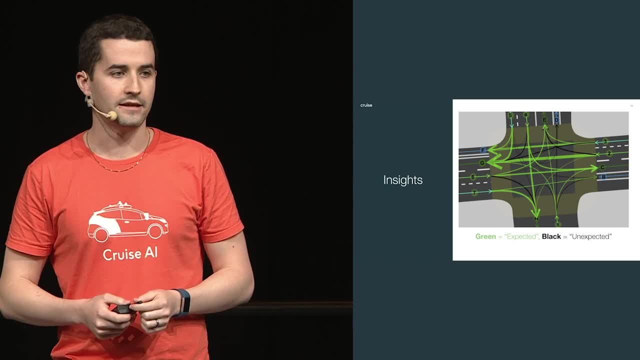 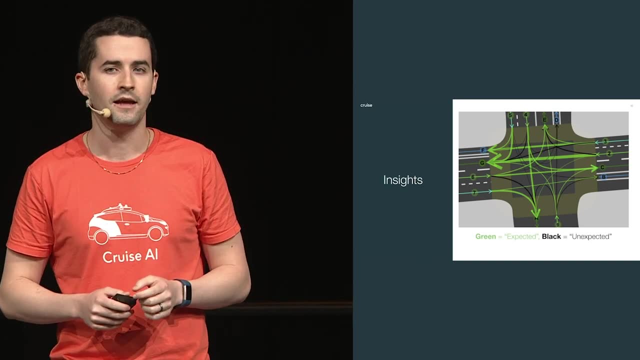 And then the thickness of the arrow is how frequent it is, And so, as you can see, there's lots and lots of black lines here of people doing basically every combination of sort of unexpected maneuver there, And so we aren't able to just assume people follow the law, especially in downtown San Francisco. 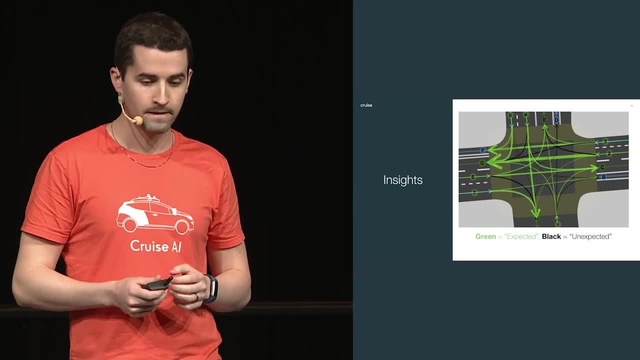 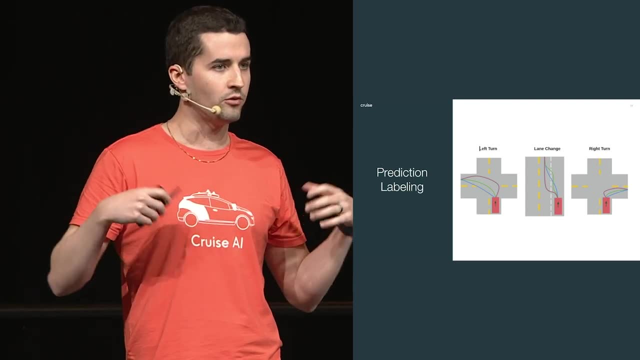 People, people drive kind of how they, how they feel they feel like it. Okay, So the last part, then, of our data set is about labeling it And so, being that we want to phrase this as a classification problem, we have to generate 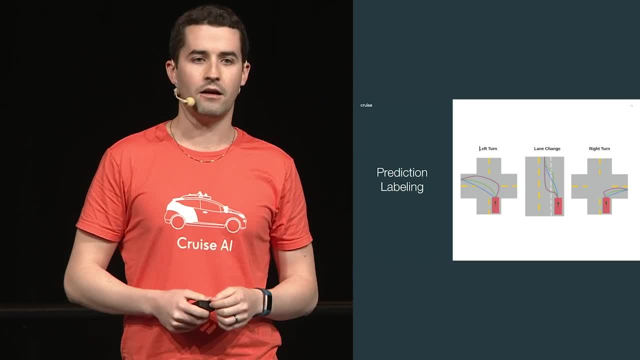 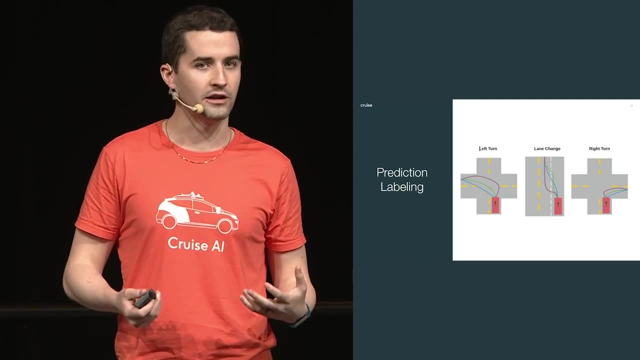 labels, And the exciting thing about the prediction problem is that we don't necessarily need a human to generate labeled data for us. If you think about trying to predict is this car going to turn left or go straight, if we wait five seconds and we see what this 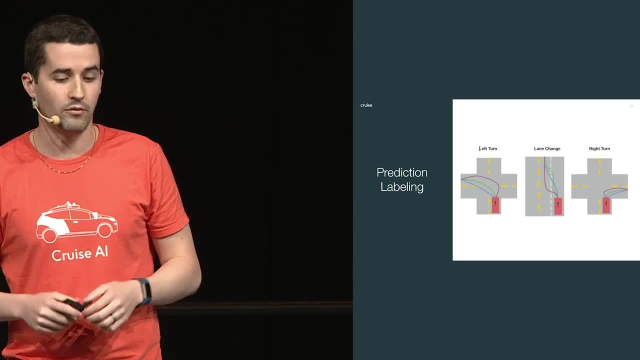 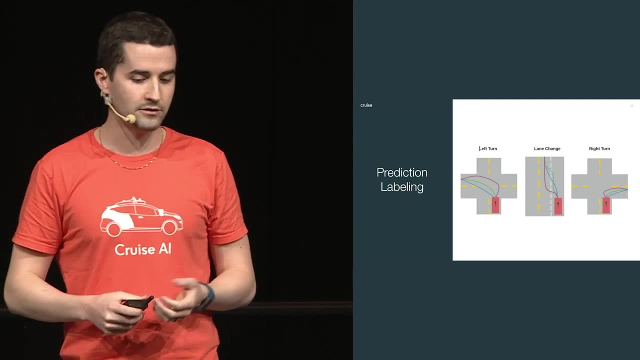 car does, we can say, oh, it made a left turn, And we can watch what they're doing. We can use our future perception information to label our previous predictions, And so what that means is not only can we build a large and diverse data set, we can label it all. So 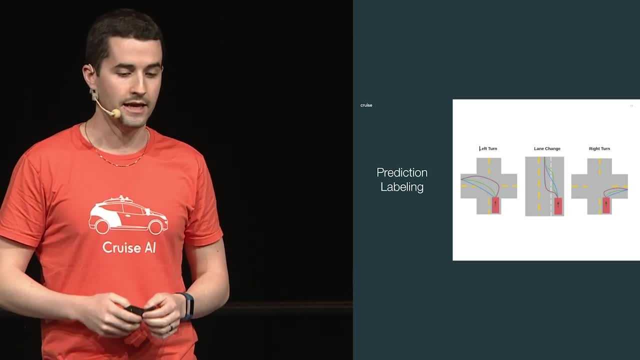 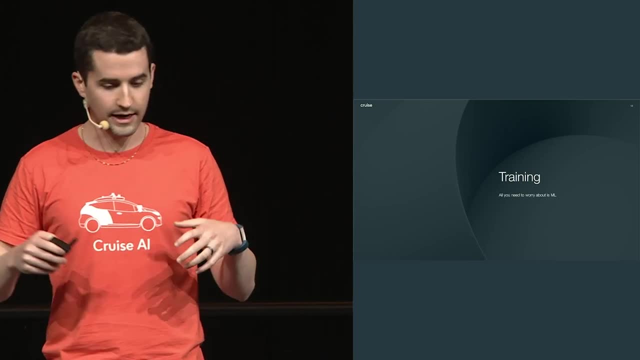